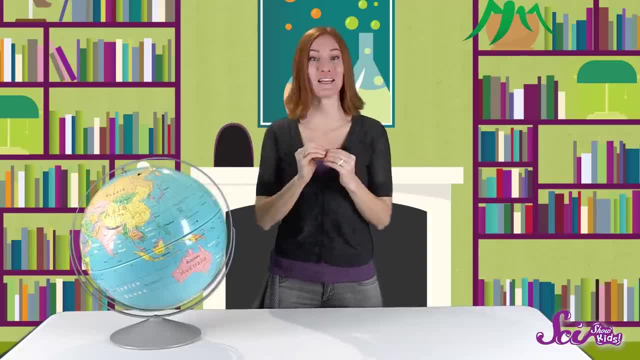 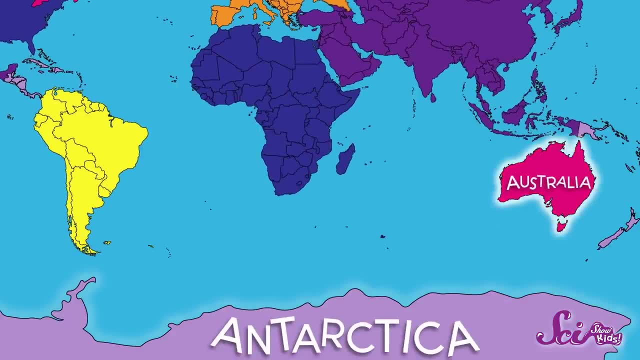 Antarctica. Most of our seven continents are divided into smaller pieces of land called countries. That's what all these different colors are within the bigger chunks of land, Like in North America, but Australia and Antarctica, Antarctica are continents that aren't broken up into smaller countries. The other five 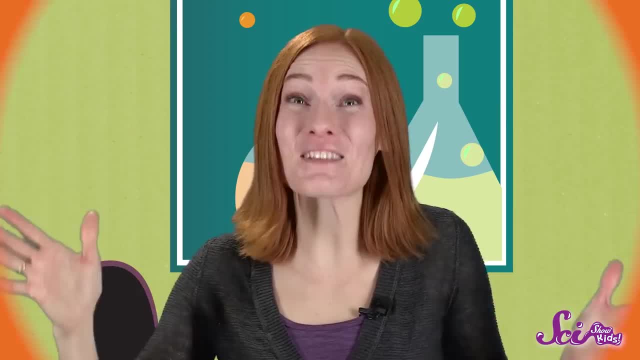 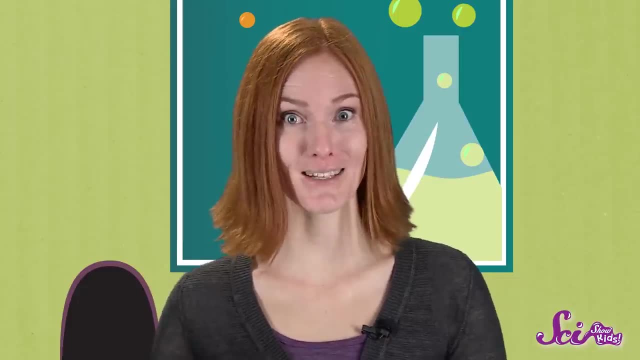 continents have almost 200 countries on them. That's a lot of land, But what's all the water on the globe? If you think there's a lot of land on Earth, just wait until you hear this: More than half of our world is covered in water. 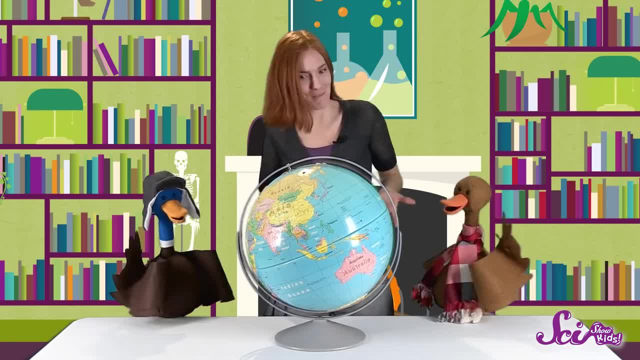 Ahem, Oh, hi Webb and hi Bill. What are you guys up to? Well, Jessie, we heard you were going to be talking about water, and who better to help you than a couple of ducks who, I don't know, live in it? 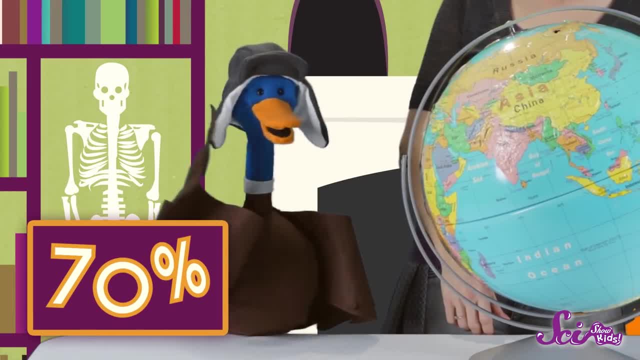 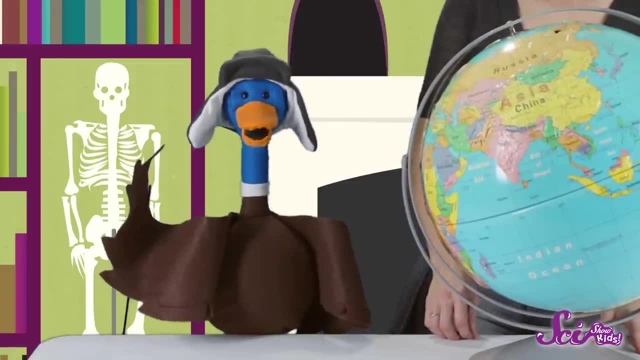 Good point. Actually, more than 70% of the world is covered in water. You're right, Isn't that cool? Some of it's freshwater, like what you find in lakes and rivers where we hang out Uh-huh, And by far most of it's saltwater, like what fills the oceans And our planet. 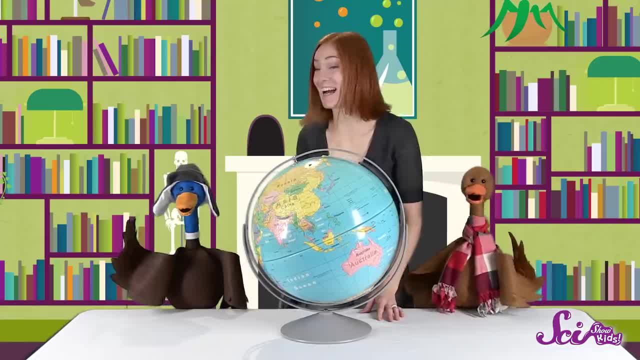 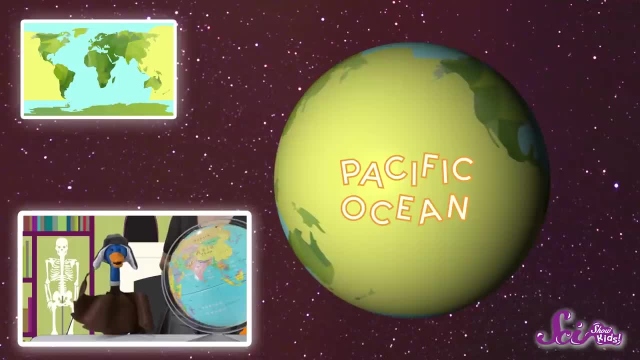 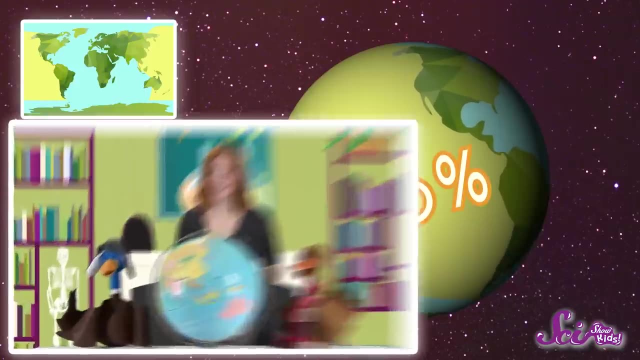 is covered in five main very big oceans Exactly. And can you name the five oceans? Of course we can. First there's the Pacific Ocean, over there between Asia and the Americas. It's the largest ocean in the world. It covers almost 30% of the planet. 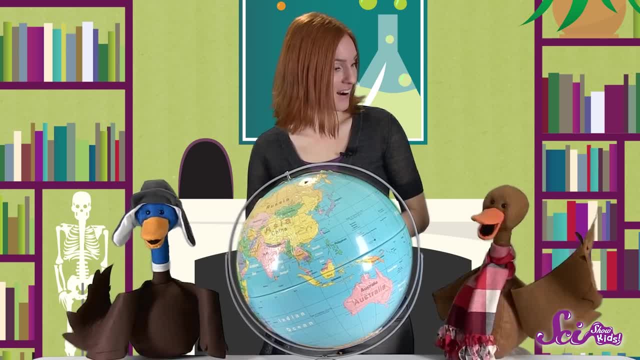 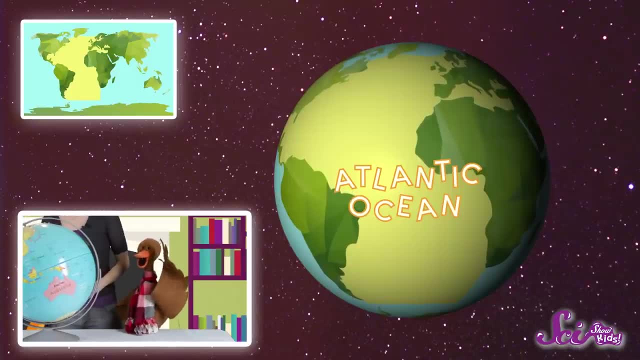 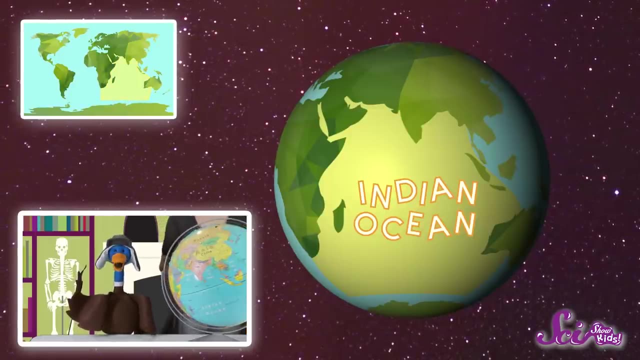 It's so big, all seven continents could fit over it, with room to spare. Whoa. But that's not all. On the other side of the Americas is the Atlantic Ocean, the planet's second largest ocean. The next biggest ocean is the Indian Ocean, below Asia and in between Africa and Australia. 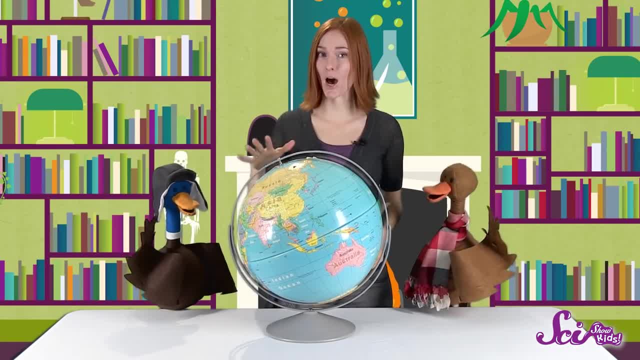 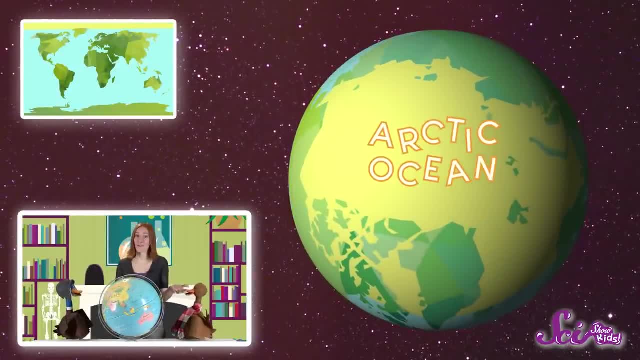 You're right. And another major ocean is up here at the top of the world, where there's no land, just water. This is the Arctic Ocean. The Arctic Ocean- Yeah, The Arctic Ocean- doesn't look much like the others in real life. That's because most 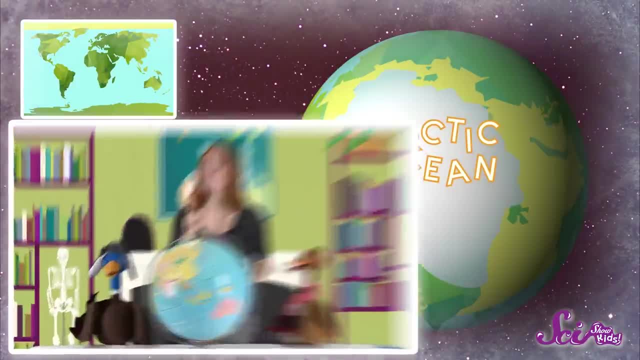 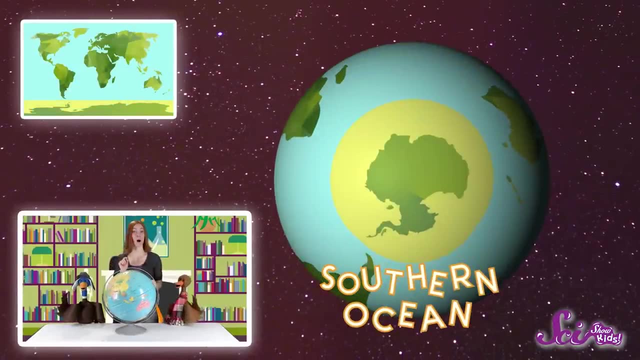 of the time it's covered in ice, Brrr. And there's just one more ocean we should mention. I know, I know, The Southern Ocean. That's right, The Southern Ocean is the name for the waters that surround all of Antarctica. 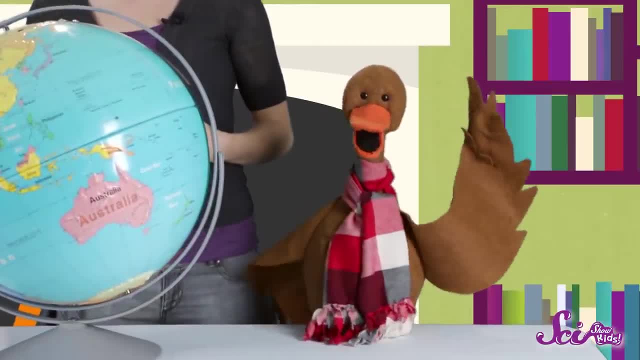 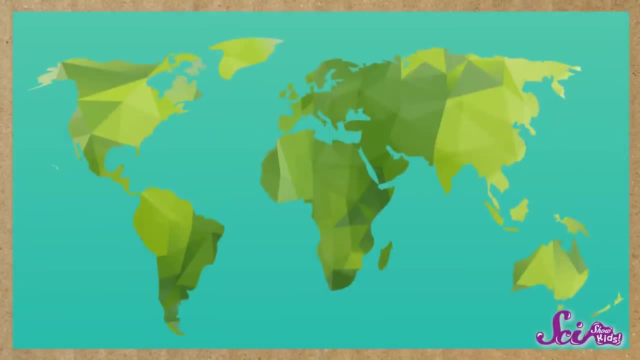 at the southern end of the Earth. I'm just going to come out and say that that's too cold for me. Me too. We're not penguins Now. we know our globe, or at least the basics of it. The fact is, there are thousands of